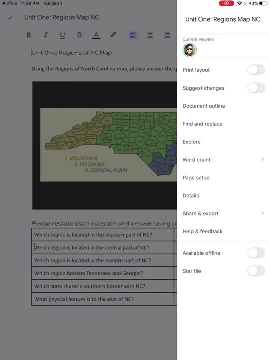 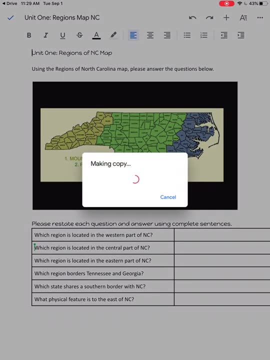 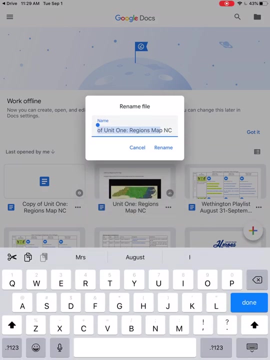 do the same. So you come up there to the three dots, click share and export, make a copy. Once you've made your copy, go back out, click rename and then all right. I'm just going to rename it the long way rather than try to get it. 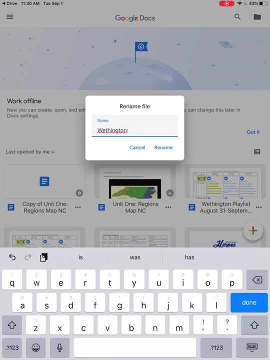 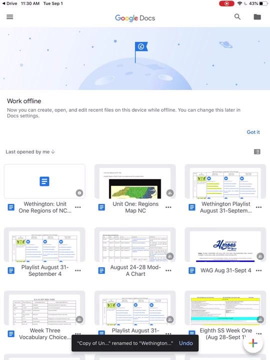 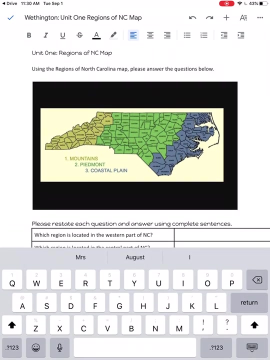 to cooperate. So it should have your first and last name, Unit 1, Regions of NC Map. All right, so we've renamed that And we'll get started. So if you look here, I've posted a map of North Carolina and it has the three main. 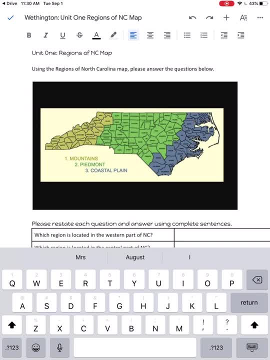 regions, which are Mountains, Piedmont and Coastal Plain, Depending on who you ask and who you talk to. there's kind of been an ongoing debate if there are three regions of North Carolina or four regions of North Carolina For the longest time I was on team. four regions just because. 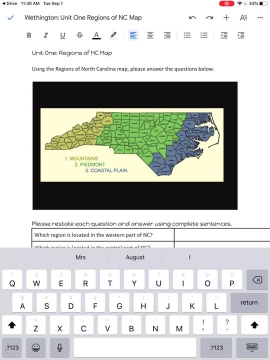 the Tidewater region- or sub-region, excuse me- is so unique and unto itself that a lot of people consider Tidewater to be its own region. However, as far as what the state recognizes for regions, usually you just have the three regions and traditionally you only have the three regions. 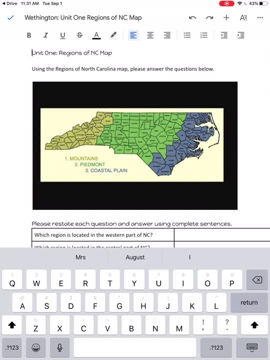 Like when I was in middle school, when I went through North Carolina history, they were still teaching the three regions. So, although I believe that Tidewater deserves to be its own region, it is not. It is just a sub-region of the Coastal Plain. So to the westernmost part of the state. 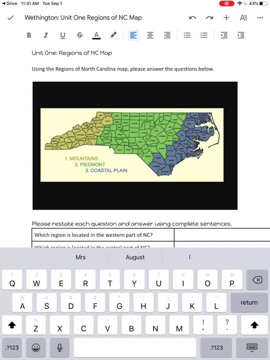 you have the Mountains or the Mountain region. It's not I, whomever, I grabbed this off of Google. It's not Mountains region, It's Mountain region. So I don't have markup open, but it would be cool if you could just take the S off of Mountain And then you have Piedmont and Coastal. 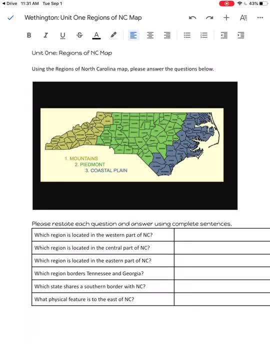 Plain. So down here. which region is located in the central part of North Carolina? You can see here in the middle the green. that's the Piedmont. The Piedmont is known for its rolling hills, Like if you look here at the map and if you're driving on 70 going. 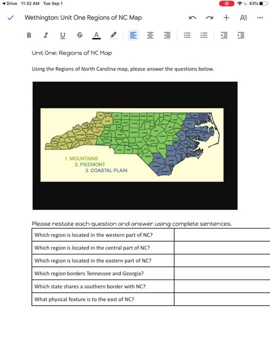 west, you'll start to notice the land getting like the hills When you get around Johnston County you'll notice it a little bit By the time you hit Durham. Chapel Hill is very the hills are very prevalent. It's definitely an elevation change. And what region is located in the eastern? 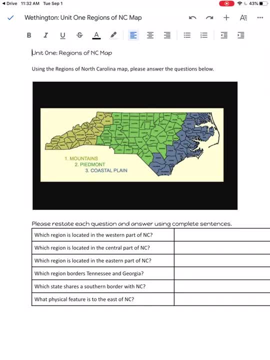 part of North Carolina, That would definitely be the Coastal Plain. So that's the Piedmont Where we live. well, actually we live in the Tidewater subregion of the Coastal Plain. The Tidewater subregion is anything that touches the water, like the ocean, And since Craven County is right there, 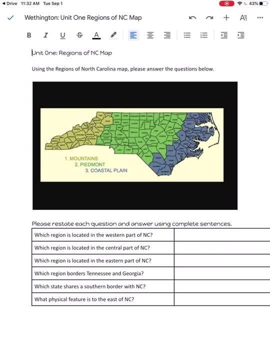 where Neuse River opens up, going towards the ocean, we are on the edge of Tidewater, So definitely Craven County and anything more eastward would be the Tidewater subregion, Which region borders Tennessee and Georgia. That would be the mountains and maybe a tiny bit into the 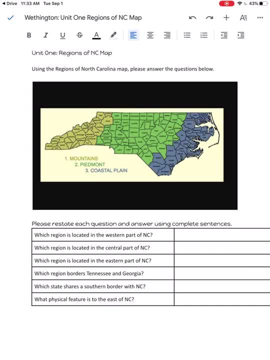 Piedmont. Most people don't know this, but there is a little place on where, like mapping, the cartographers that created the maps of the states. They drew in a little bit and I don't have a map to show you right now. I'll show you tomorrow where you can look it up. They drew the map for 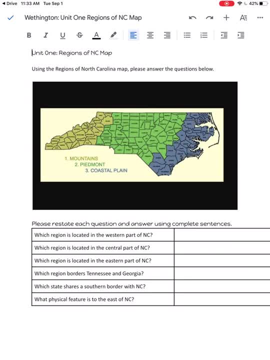 Georgia in just a little bit to where North Carolina actually borders Georgia. So that's a very small space. So we have Virginia to the north of us, We have Tennessee to the west, South Carolina to the south and a tiny bit of Georgia to like the southwest. What physical feature is? 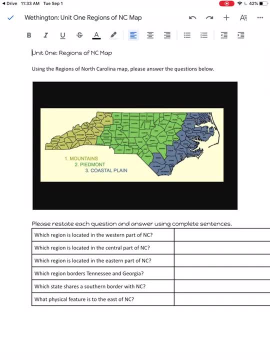 to the east of North Carolina. If you remember me just talking about Tidewater and it being attached to the ocean, that would mean the Atlantic Ocean is the physical feature. that is, to the east of North Carolina. As we go over the individual regions and their respective subregions, we'll talk. 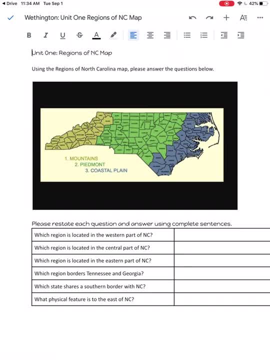 more about what each region has to offer, But as far as looking at a map and finding the three main regions of North Carolina, that's what you need to know for this assignment. So, now that we've talked about it, what I need you to do is go in and answer the questions below. You will restate: 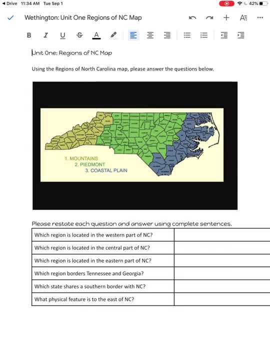 each question and answer using complete sentences. If you are unsure as to how to restate the question, you can go ahead and do that. You can go ahead and answer the questions below. You will restate each question and answer using complete sentences If you are unsure as to how to restate the question. 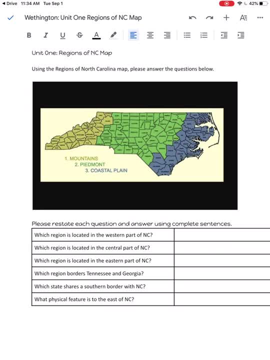 you can go ahead and answer, use complete sentences If you are unsure as to how to restate the question. So if you would go on and get started working on this and turn it into the August 31st North Carolina Regions assignment on Canvas, which you can access by using our playlist If you have any. 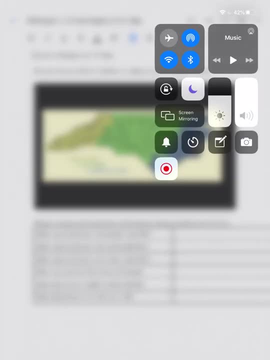 questions, as always. please email me and have a good day. 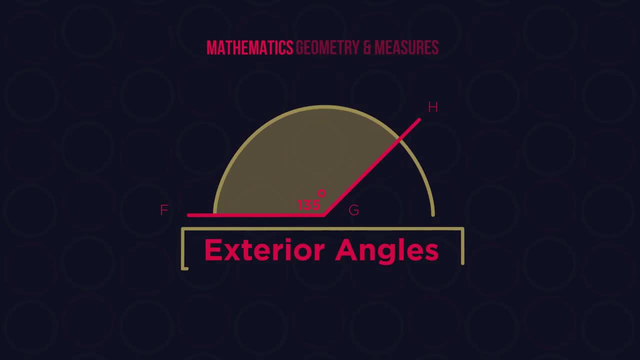 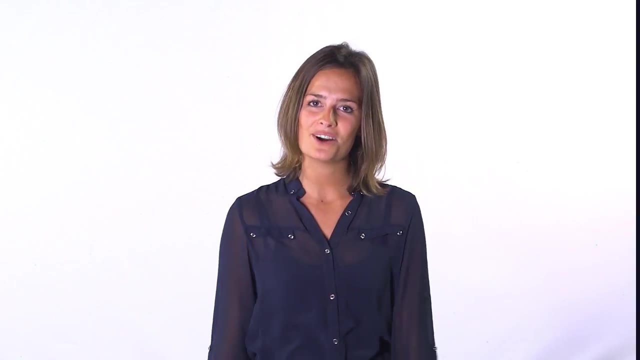 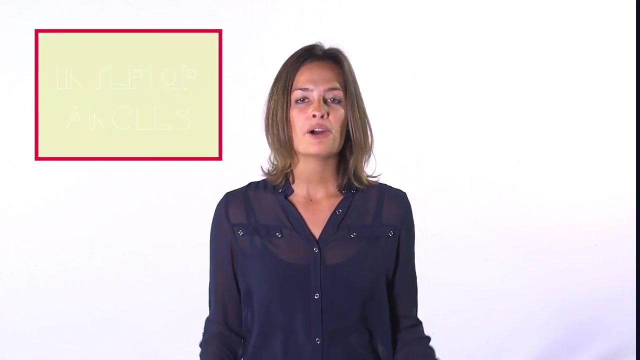 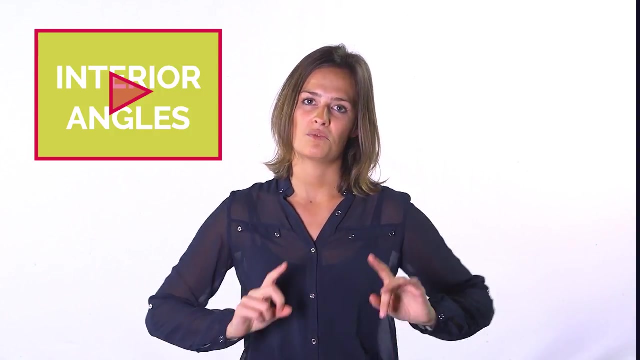 In this video we're going to look at the exterior angles of polygons: Firstly, what they are and secondly, the sum of exterior angles. We looked at interior angles in another video. We looked at the sum of interior angles and the size of one interior angle. If you're unsure about them. 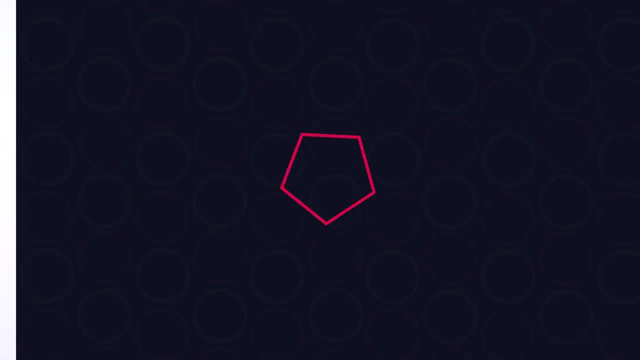 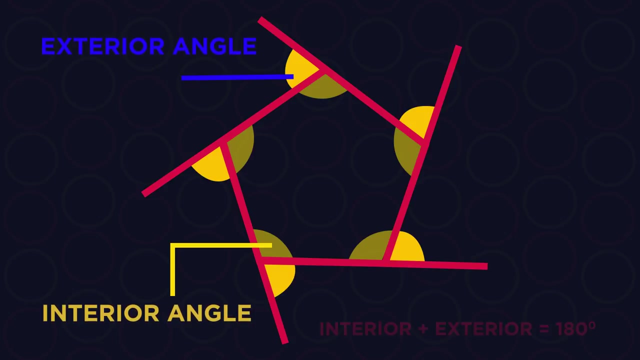 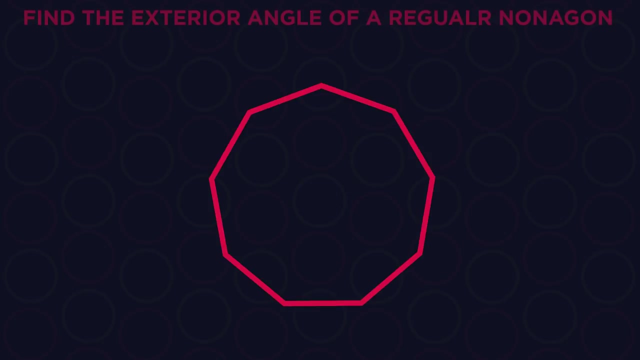 you may want to watch that video first. So let's have a look at exterior angles. They're a little strange. Exterior angles make a straight line with the interior angle. They aren't the whole outside angle, but just the part that makes a straight line. What's the exterior angle of a?